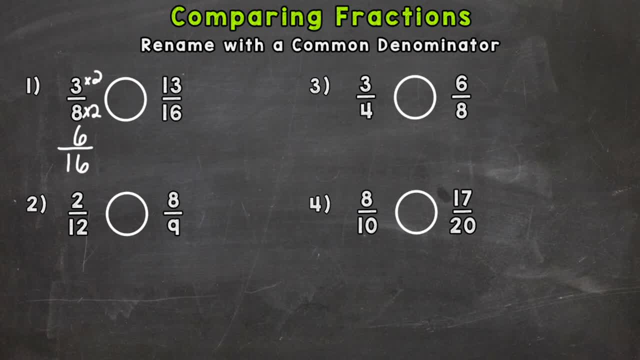 problem. I just renamed with that common denominator The second fraction, 13, 16, already has a denominator of 16. So I do not need to rename or do anything to that fraction Now that we have a common denominator. It's very easy to compare And we can see that. 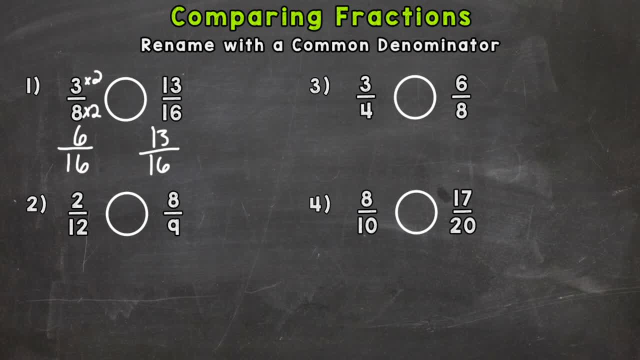 6- 16th is less than 13. 16th Right, 13 out of 16 is going to be greater than 6 out of 16.. So let's put our symbol in here And we can read that from left to right: as 3- 8 is less than 13- 16.. Another way to think of this problem is: you can see, on the left We have 3 eighths Right. That is 0, 9, 8, 8.. Now they are a ball. So if you just put this in here and you add 1, 8, 8, you'll see that. 0, 8, 8 is a söylena for 9, 16.. So I don't have the front 6, 7.. Those operations are missing by 3, 8. It doesn't have to be as tight as that one, but you can see that the problem is. you can see on. 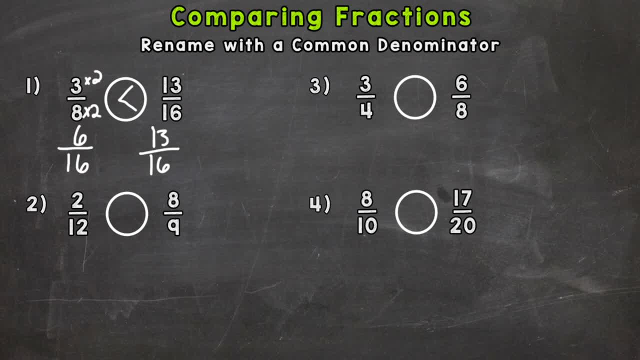 e, f, 3 eighths right, That's less than 13, 16 right. So another way to think of this problem: right, that's less than half, because half is 4 eighths. so the left side is less than half. now, on the right, we have 13, sixteenths and that's greater than a. 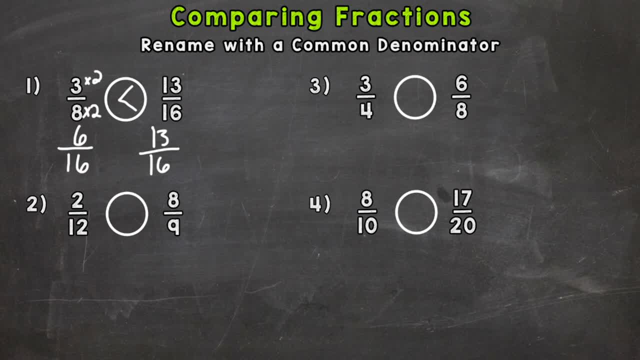 half, because half of 16 is 8 sixteenths, so the right side is more than half and the left side is less than half. so we could tell by using that strategy, or you can prove it by changing the denominators, you know, using a common 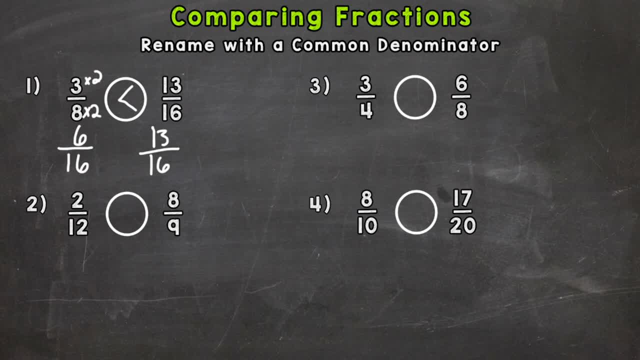 denominator and renaming. so let's take a look at number two. here we have two twelfths and eight ninths. we do not have a common denominator, so let's find one and rename. so for 12 and 9, your common denominator is going to be 36, 12 times. 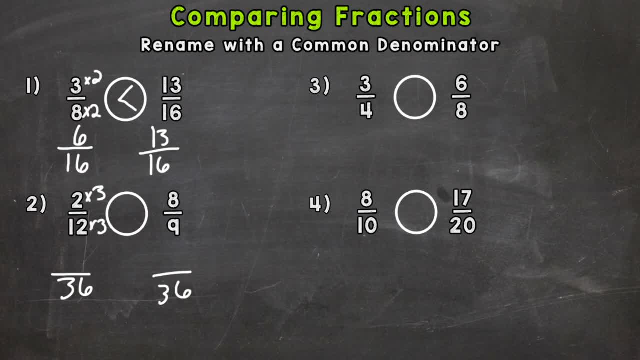 3 is 36, and so let's do the same thing to the top. 2 times 3 is 6. 9 times 4 is 36. so do the same thing to the top. 8 times 4 is 32, now that we have a common denominator. 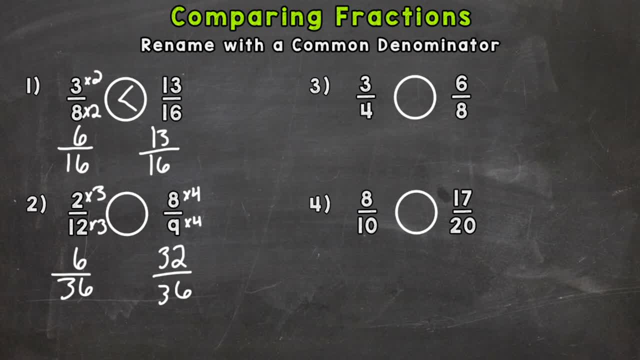 and we renamed. it's very easy to compare: 6, 36 is less than 32, 36, exactly. so take a look at 1, 9, 12, right side. again, do the same thing for 2, 9, 9, 12. so now, when you have a common denominator and wrench, there will be 0. 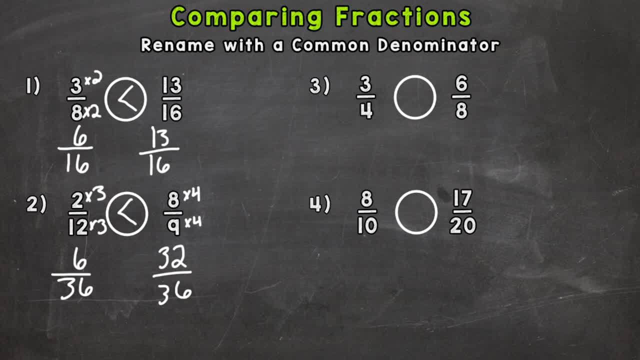 it is 5. so if it's leaving the denominator 2, get out of thisgreen denominator, since our denominator of 9, wad or point, then it is abroad. hip ł to the left. now let's take a look at the original problem again. now, 2, 12th. 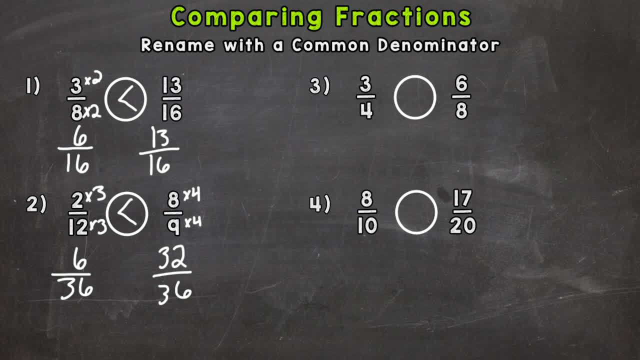 is less than half right, because 6 out of 12 is half. so obviously 2 out of 12 is less than 6 out of 12. so the left side is less than 1 half and the right side half 1-9. we have 8 ninths, so we're well over. half. so the right side, right off the bat, we'll put it in particularly this part- and the snake goes up. and then we have 1 divided by 1angle, because it Dann Lee's hem, 6 out of 12 later and he's isn't half. and then we have 8, ninths, 6 and 9 in theignon. 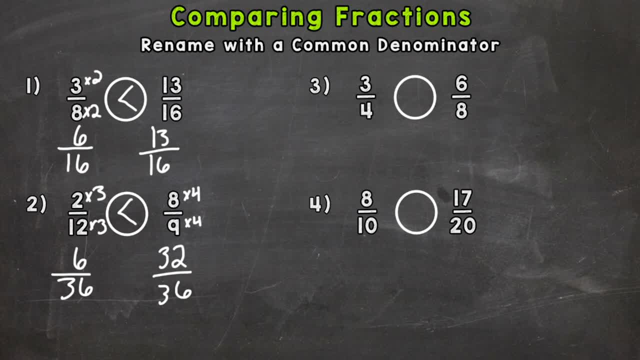 Right off the bat we could see it's more than half and the left side is less than half. That can also help us compare. But again, we proved the comparison when we found a common denominator and renamed. So let's take a look at number three. 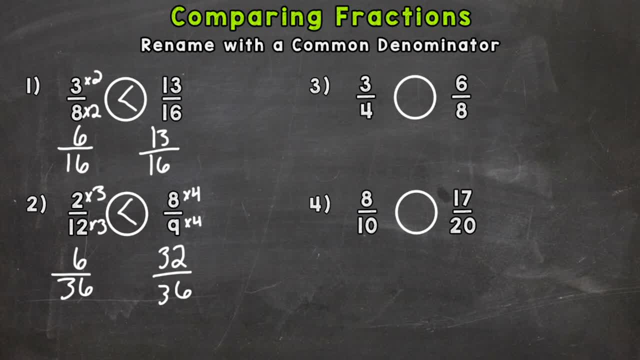 Now both of these fractions are over half, so we can't use the benchmark strategy here with these fractions. So we're going to need to find a common denominator and rename So three-fourths and six-eighths. So we have a four and an eight and our common denominator is going to be eight. 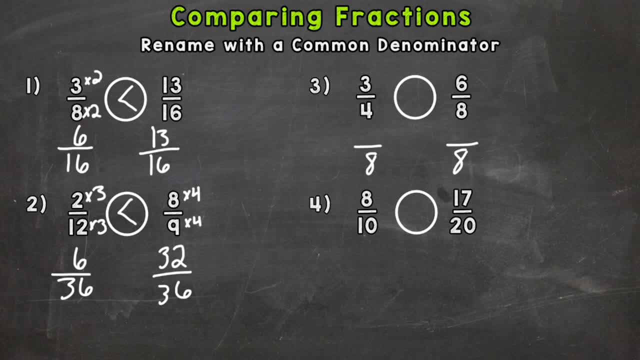 Now that second fraction, six-eighths, already has that denominator of eight, so we do not need to do anything. We're going to leave it as is. Three-fourths. okay, we need to think. well, four times two gives me that denominator of eight. 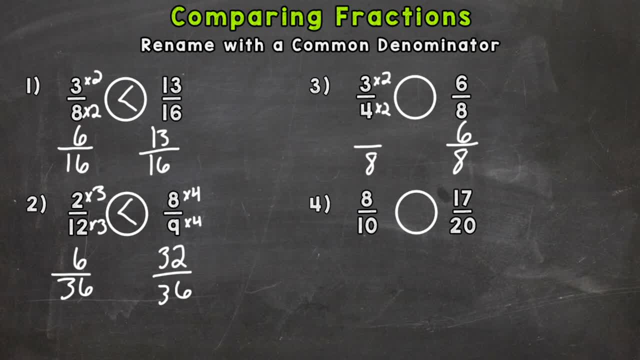 so I need to do the same thing to the top. Three times two Gives me six. So both sides are equivalent to six-eighths. So both these fractions are equal. So three-fourths is equal or equivalent to six-eighths. 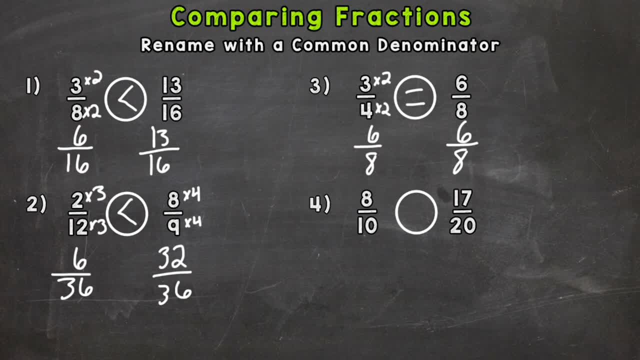 Let's take a look at number four And just using benchmarks and fraction sense when I talked about the half for numbers one, two and three. that's a benchmark fraction. That's a fraction that we can base different things off of. 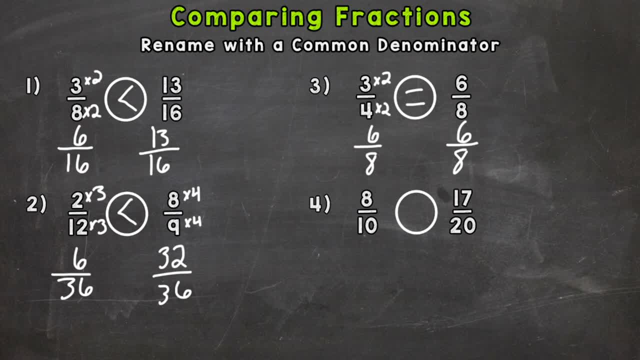 So when I say the word benchmark, I'm just talking about a fraction we can use to help us through these problems. Now, eight-tenths is above half right, because half would be five-tenths, And on the right we have seventeen-twentieths. 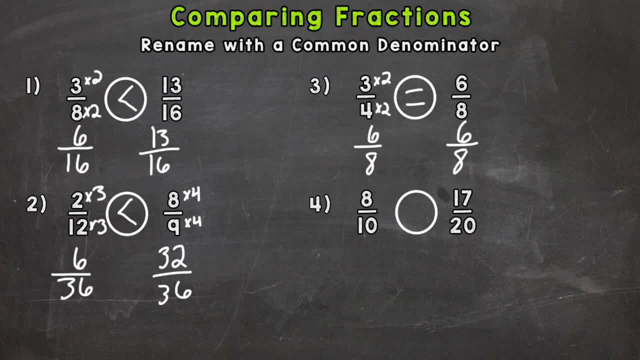 Well, half a twenty is ten, So that one's above a half as well. So we can't really tell right off the bat which one's greater or less than So let's rename. Let's rename with a common denominator. So we have a ten and a twenty.